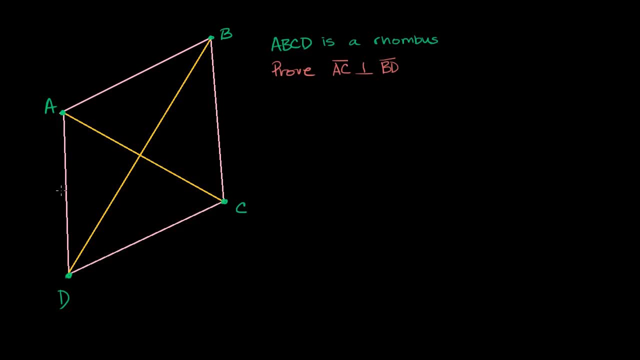 of a parallelogram. In a parallelogram the opposite sides are parallel, So that side is parallel to that side. These two sides are parallel. And in a rhombus not only are the opposite sides parallel- it's a parallelogram- but also all of the sides. 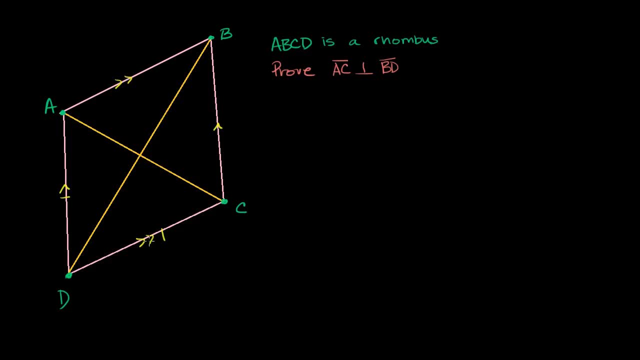 have equal length. So this side is equal to this side, which is equal to that side, which is equal to that side right over there. Now there's other interesting things we know about the diagonals of a parallelogram, which we know all rhombi are parallelograms. 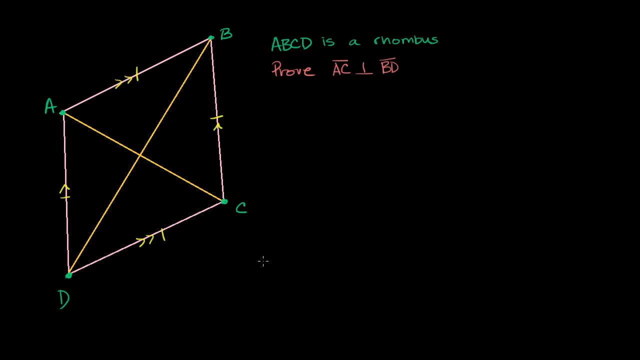 The other way around is not necessarily true. We know that for any parallelogram- and a rhombus is a parallelogram- that the diagonals bisect each other. So, for example, let me label this point in the center. 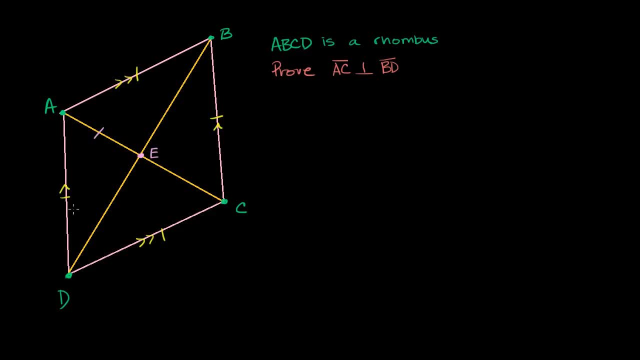 Let me label it point E. We know that AE is going to be equal to EC- I'll put two slashes right over there- And we also know that EB is going to be equal to ED. So this is all of what we know. when someone just 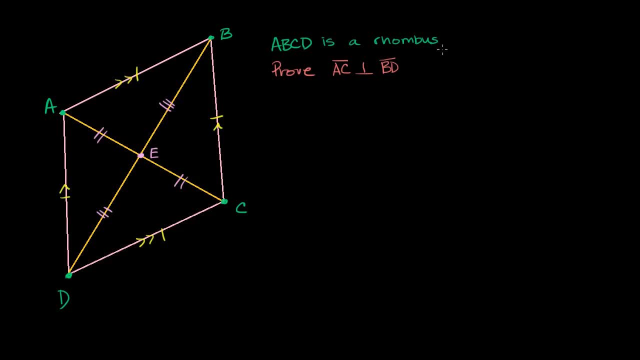 says that ABCD is a rhombus, based on other things that we've proven to ourselves. Now we need to prove that AC is perpendicular to BD. So an interesting way: Let's prove it And you can kind of look at it just by eyeballing. 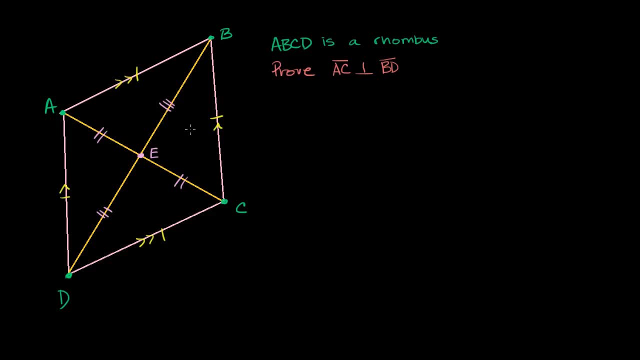 Because if we can show that this triangle is congruent to this triangle and that these two angles right over here correspond to each other, then they have to be the same and they'll be supplementary, and then they'll be 90 degrees. 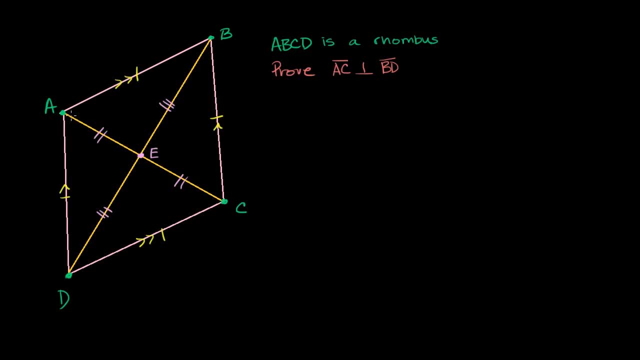 So let's just prove it to ourselves. So the first thing we see is we have a side, a side and a side, a side, a side and a side, So we can see that triangle. let me write it here. 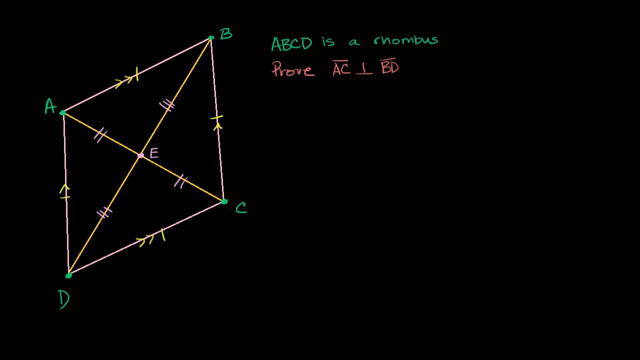 triangle. let me just do it in a new color. We see that triangle, Triangle, triangle ABE is congruent to triangle CBE And we know that by side side side congruency, We have a side a side and a side, a side, a side. 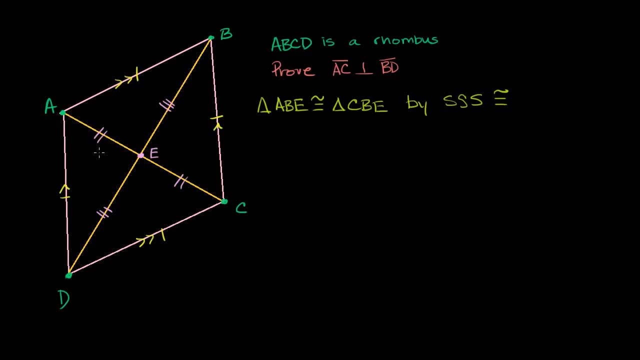 and a side. And then, once we know that, we know that all the corresponding angles are congruent And, in particular, we know that AEB, we know that angle, ABE, Angle, AEB is going to be congruent to angle.